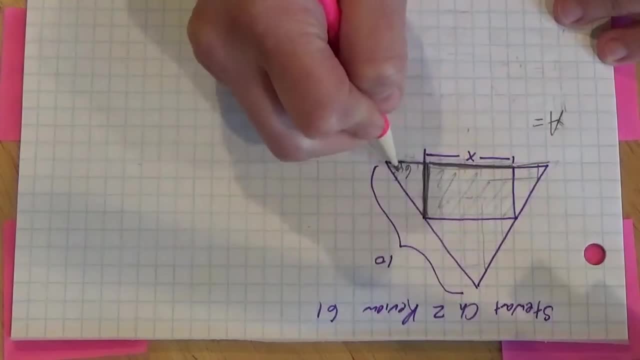 Now they tell me it's an equilateral triangle. so then I know that all the angles are 60. And so, since the height is at a right angle, this is a 30-60-90 triangle. So that's going to help me find the height, as long as I know what this side is. 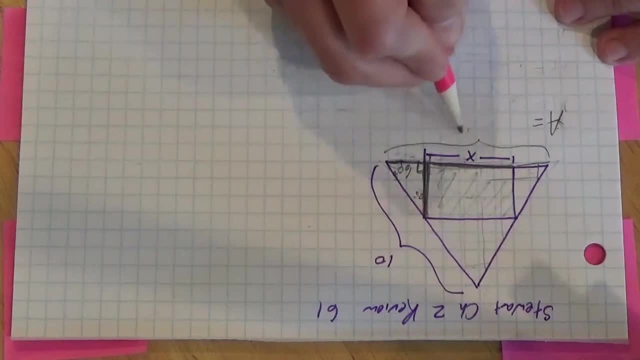 Now this little length here. it's not the full 10, nor is it 10 minus x. If I did 10 minus x, that would give me what's left here, Like if x were 6, then I'd have 4 left in here. 2 and 2, right. 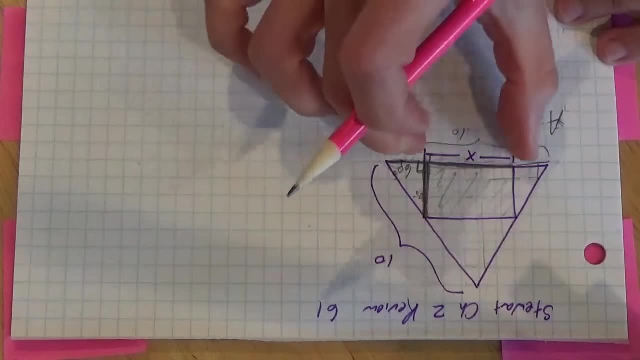 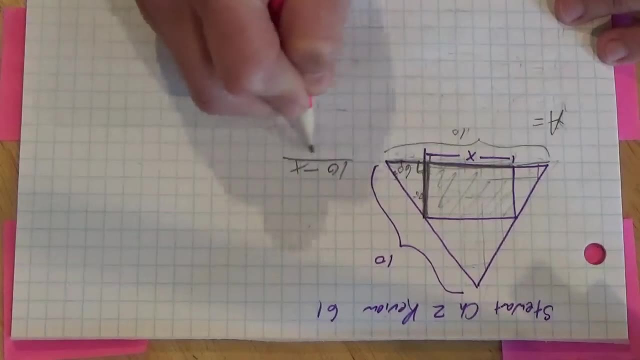 Or if x were 4, then I'd have 6 left for here, 3 and 3.. So what this little length is going to be, it's 10 minus x divided by 2.. So I'm going to write this as 10 minus x. 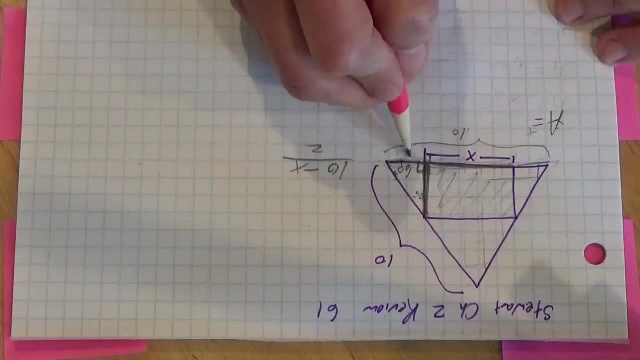 So I'm going to write this as 10 minus x. So my area and that's oh, so this little part here, is 10 minus x divided by 2, and that's the shorter leg of this 30-60-90 triangle. 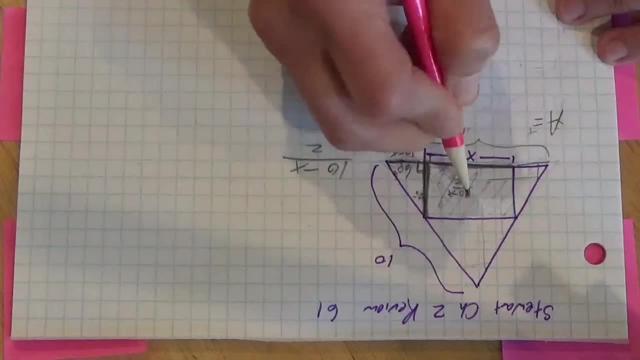 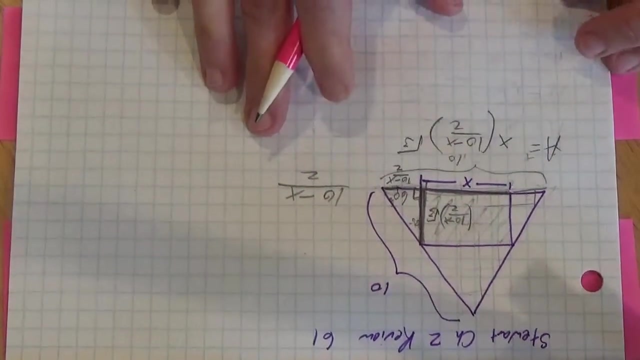 So the longer leg is 10 minus x over 2 root 3.. So that's the height. So my area is the base, which is x times the height, 10 minus x over 2 root 3.. Excellent, So we have a. 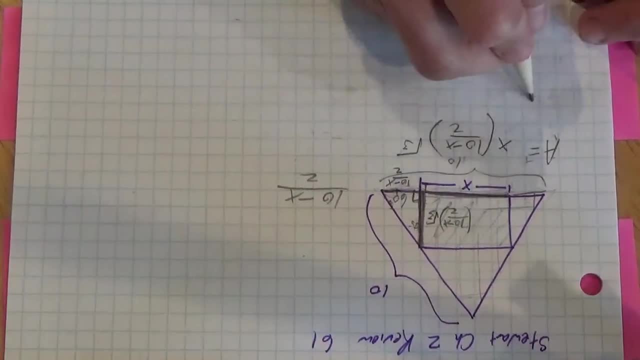 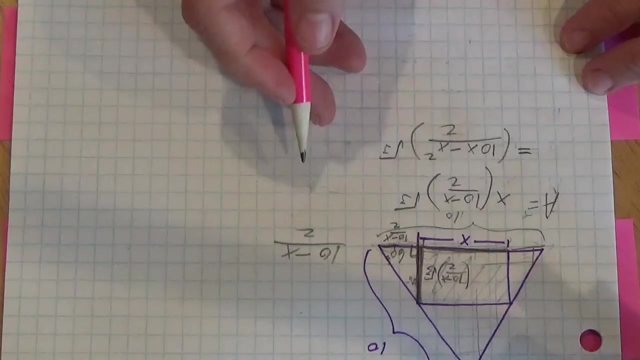 So we have a formula for area all in terms of x, And I could make it a little bit cleaner. What if I went ahead and distributed the x? So I'd have 10x minus x squared over 2 root 3. And I could either distribute in the root 3 or take it out. 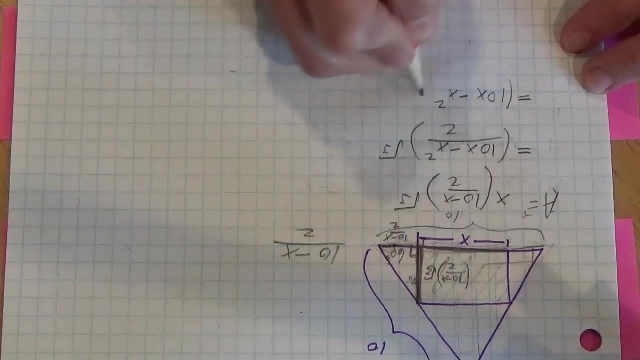 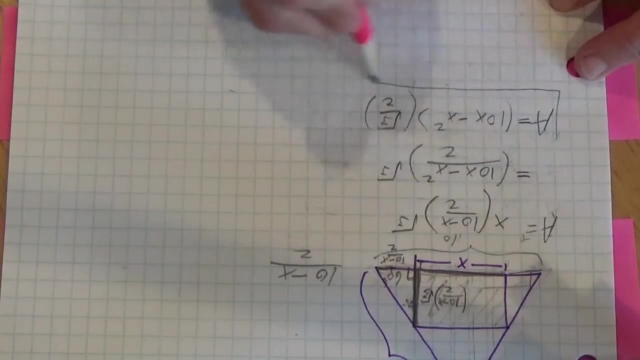 I think I want to take it out. So I have 10x minus x squared times root 3 over 2. And that looks a little bit cleaner. So there's a formula for area all in terms of x, And they also ask us to maximize the area of this. 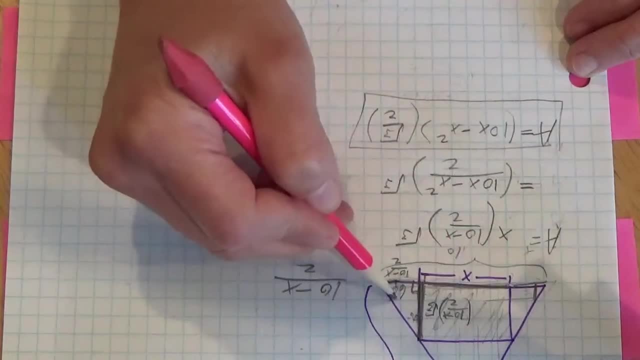 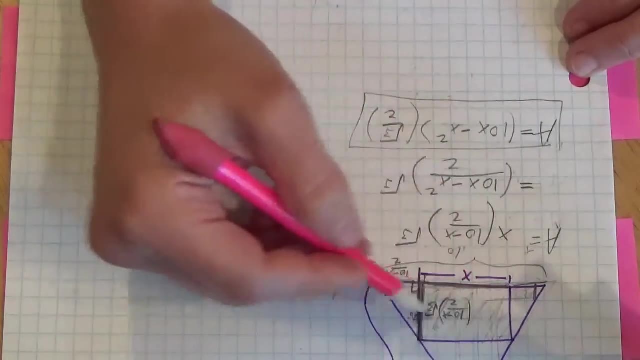 So we could have had a rectangle where x was really big and then it wouldn't have as much area, Or somewhere in the middle here, when x is about where I have it, it looks like a maximum, Because if I made the x small, 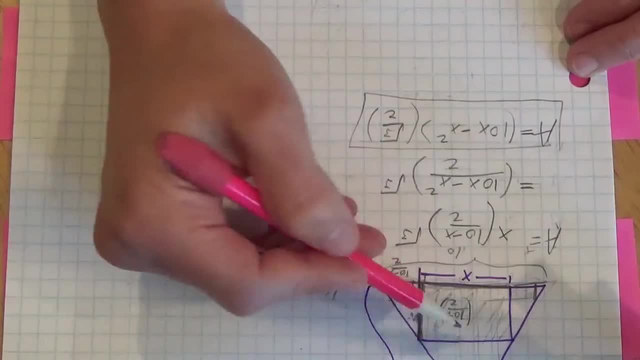 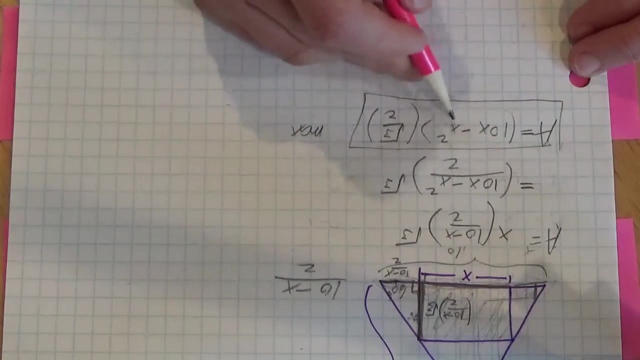 you would have a skinny rectangle with not as much area. So whenever they ask you to to maximize or minimize your, unless you know calculus, you're hoping that it's a quadratic, because its graph is a parabola, an upside-down parabola. 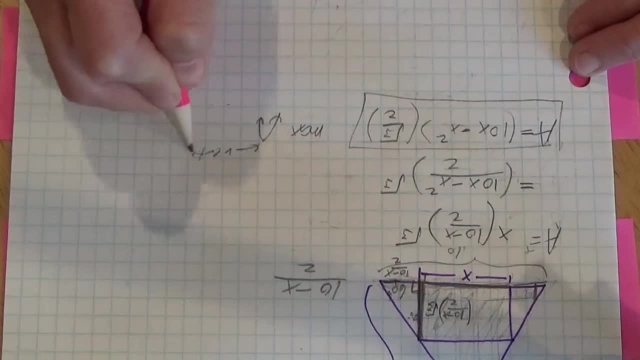 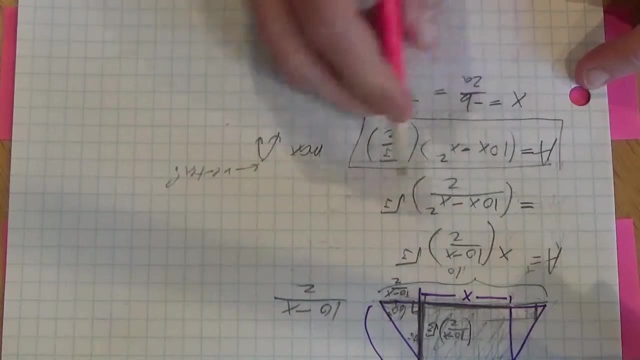 because this is negative and the max is at its vertex. So we have a formula to find the vertex: x equals negative b over 2a. So here x is negative b, which is negative 10, over 2a, which is negative 1.. 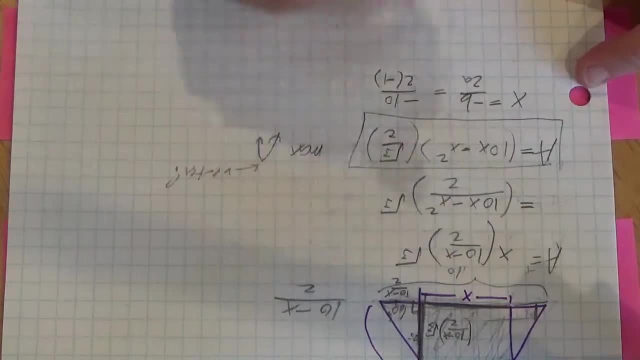 I could have put the root 3s over 2 distributed in there, but they would just end up canceling out. So it works. So we get a maximum area when x is 5. And so that'll be the x that'll maximize your area. 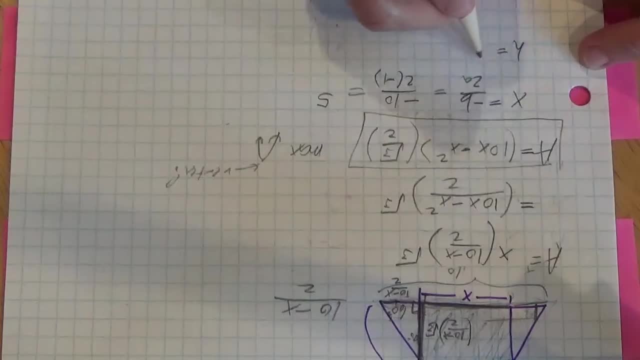 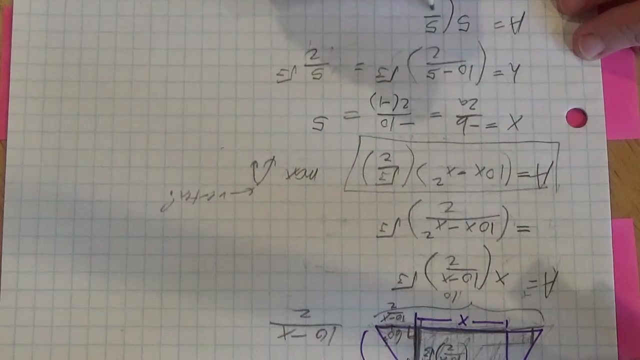 If you wanted to find out what the height would have been, the height would have been 10 minus 5 over 2 root 3.. So that's 5 over 2 root 3.. And then the area. you could have either done base 5 times height, 5 over 2 root 3,. 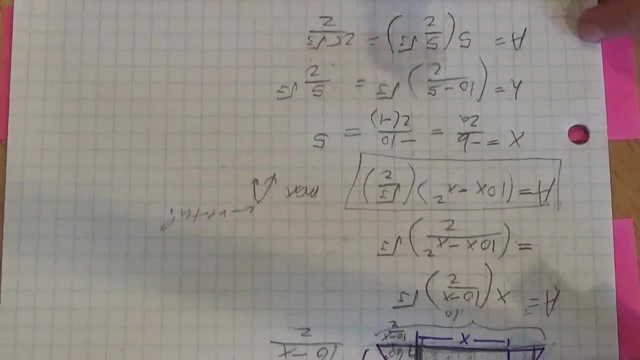 which is 25 root 3 over 2, or you could have put the x back into our area formula- any one of those area formulas- and gotten this, So that answers our question. So we have an area formula of that, a max area when x is 5,. 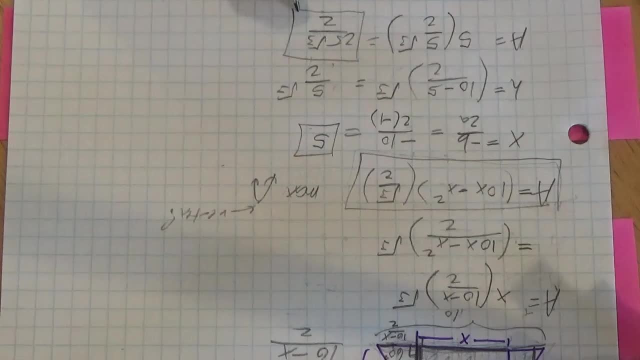 and the area will be 25 root 3 over 2.. Excellent. 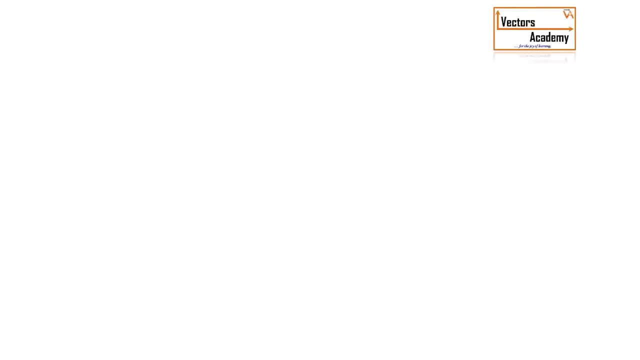 We will now study a new method to solve linear equations, That is, the graphical method. We have already studied how to draw a graph of a line. Now suppose there are two equations which are given. We will consider the first equation, that is, x plus y equal to 6.. Now